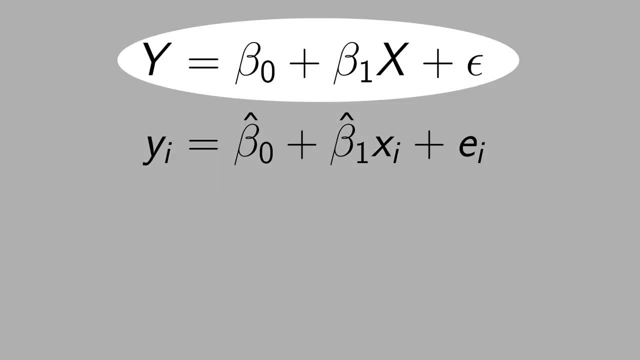 We use a different notation to distinguish the theoretical probability model from the data. The lowercase Y is the outcome variable and see the subscript I. I is the unit of Nella's observations. Now the intercept is beta, hat zero. The hat means this is estimated from data. 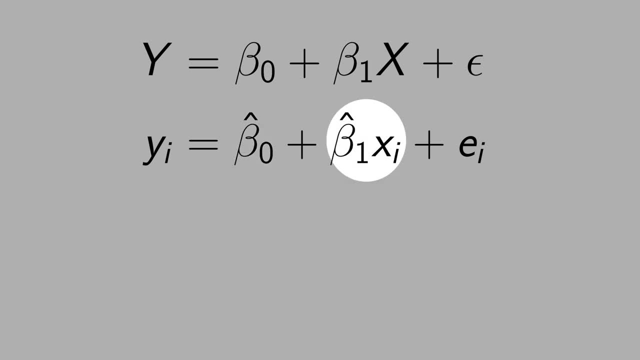 The same logic applies for beta one, hat and Xi. See that now we use English letter instead of Greek letter. When we are in the data world, we call this term as Residual rather than error term. We can isolate the residual in the right side of the equation. 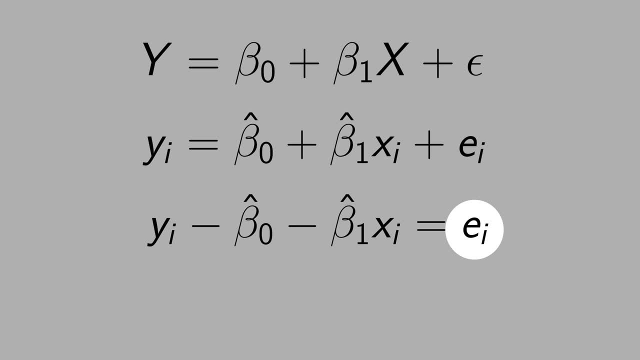 And see the logic of the name residual leftover. It is the difference between Y and the splinter variables. But the splinter variables cannot explain completely why. That's why you have the residual left over. Mathematically speaking, ordinary square is about minimize the residual sum of square. 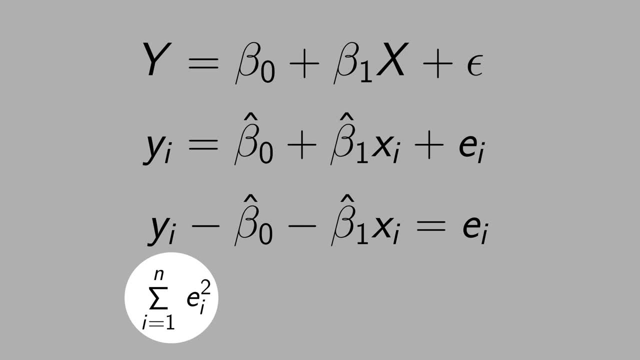 See that if you have any data points, we have any residuals, and you have to sum up all these residuals from 1 to N. And you see, that is not the simple residual, It is the square of the residuals, By definition. you just square this term here and you get the residual sum of squares. 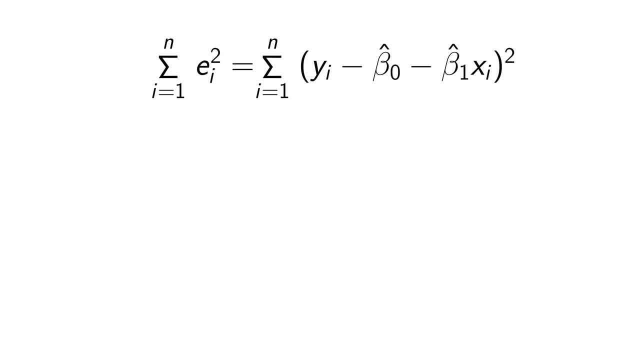 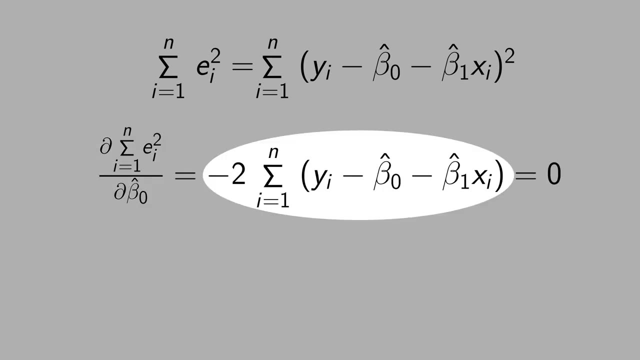 If you want to minimize a function, you have to take the derivative. Let's take the derivative of the residual sum of the squares in relation to beta zero. Here is the derivative. Let's apply chain rule. The two go outside. Then we take the derivative of the inside term with respect of beta zero. 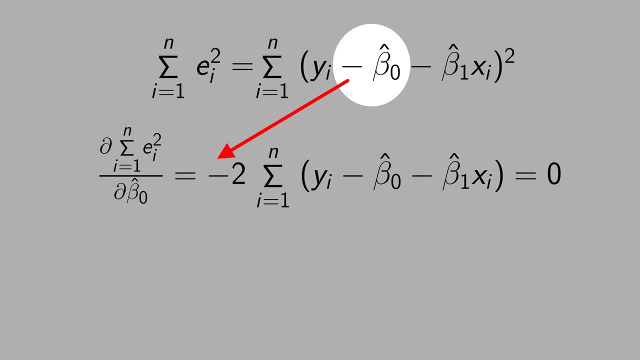 You'll be 1 and this minus will be outside of the two And you copy what is inside. We just apply the chain rule from calculus and we make the derivative equal 0 to get the minimum. If you need this term equal 0 as a first order condition. 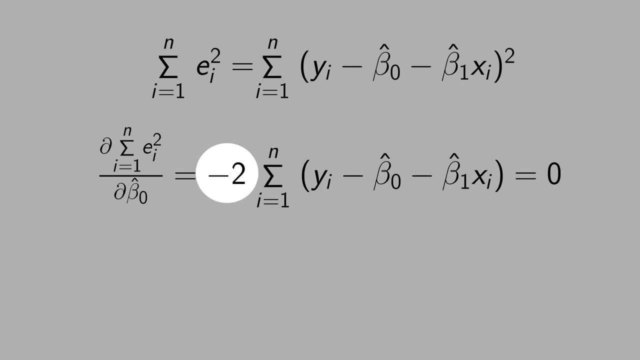 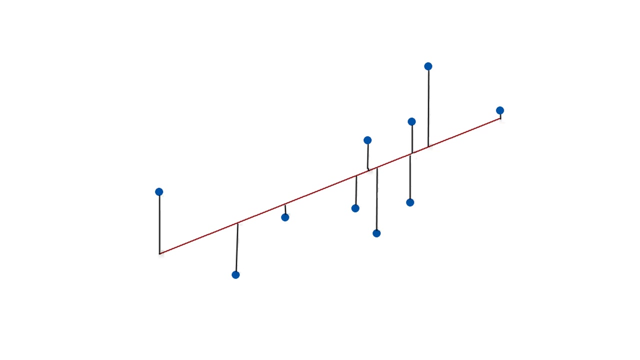 this minus 2 is my derivative two. you can ignore because cannot be zero. that means this part has to be zero and what is this part inside is the residual. therefore, the residual has to sum up to zero. this is intuitive. the residuals are these vertical lines. some residuals is above the line and the other are below the line.